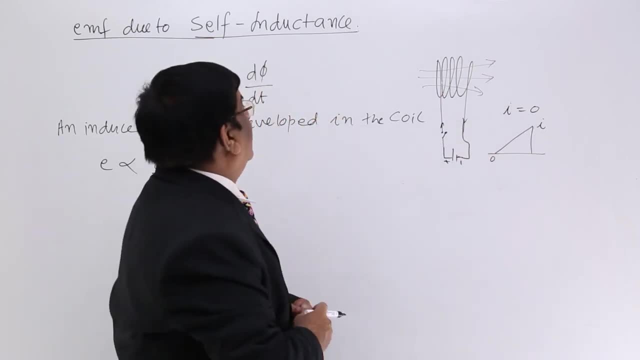 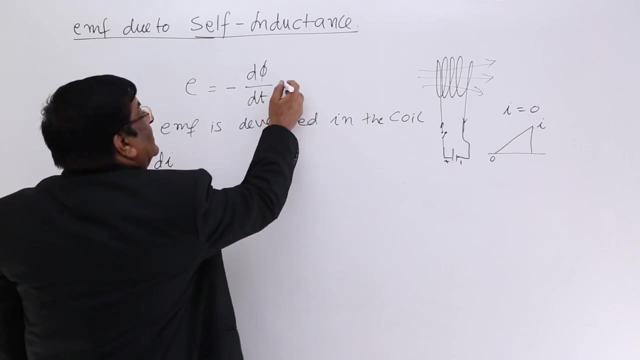 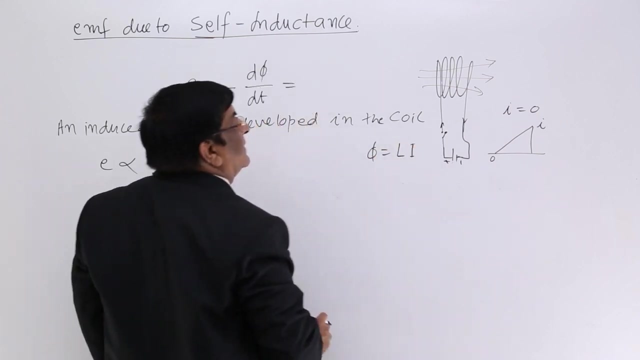 there will be change in flux and due to change in flux and EMF is induced. induced and that EMF, according to Faraday's second law, is minus d phi by dt. Now this phi. in the previous lecture you have seen that phi is equal to L into I. This is: 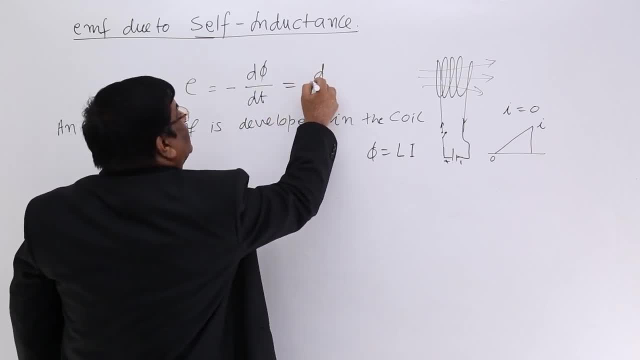 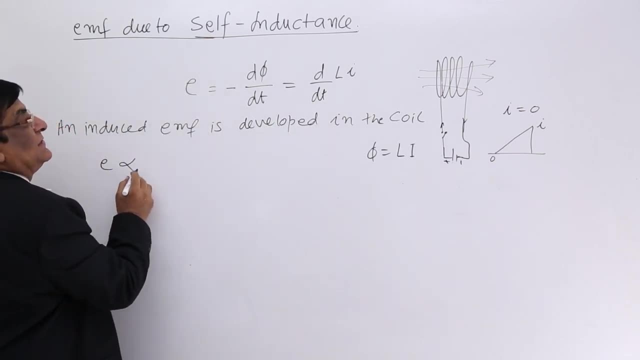 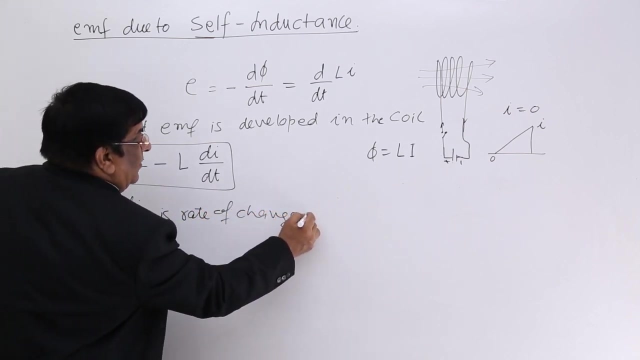 coefficient of self-inductance. This we introduce here. So this is d by dt of L into I and therefore we can write it: E is equal to minus L, dI by dt. dI by dt is what Rate of change of current? dI by dt is rate of change of current. Now suppose in a coil there is a current of 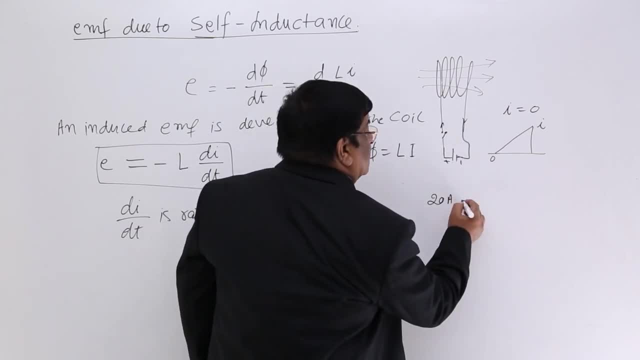 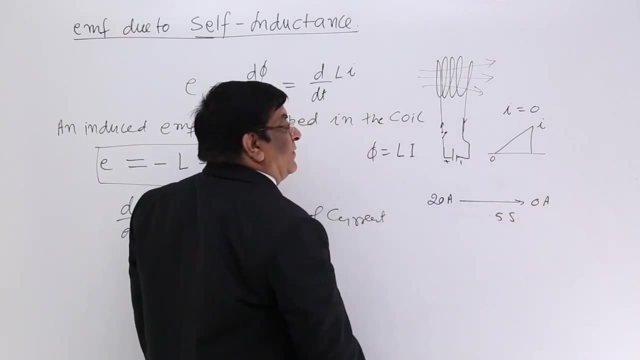 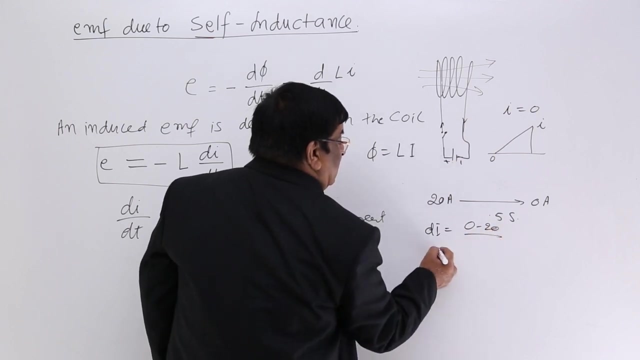 20 amperes. They are flowing and when we switch it off, this become 0 ampere, and this takes a time of 0.5 second. What is dI by dt? Answer: dI is equal to 0 minus 20.. dT is equal to 0.5. 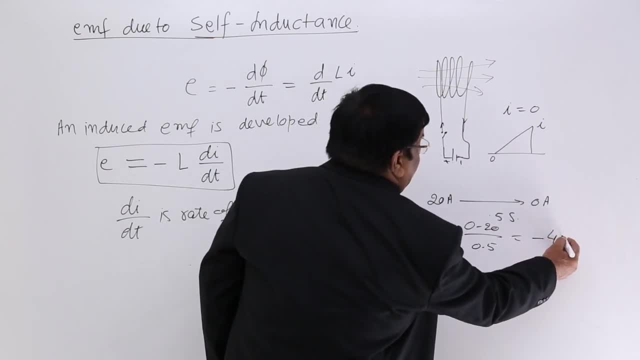 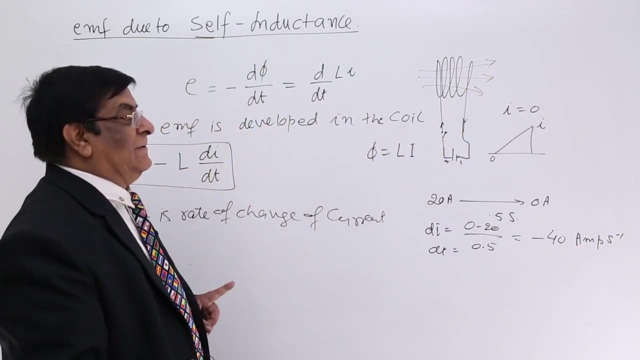 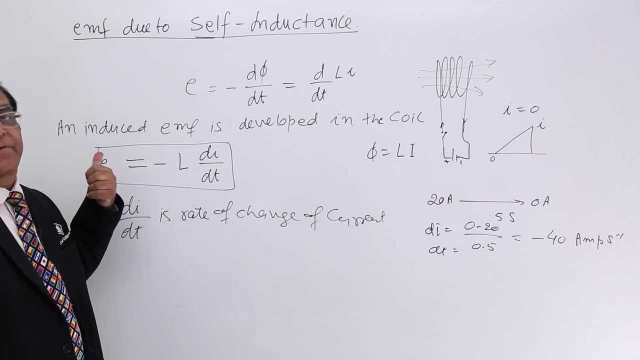 So dI by dt is equal to minus 40 ampere per second. This is example of dI by dt. More is the value of dI, more will be EMF. Less is dt, more is EMF. So this is. 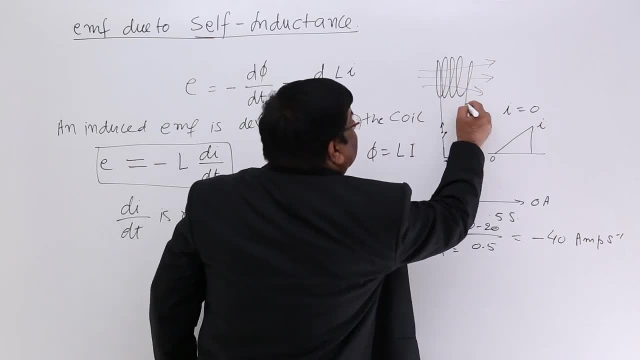 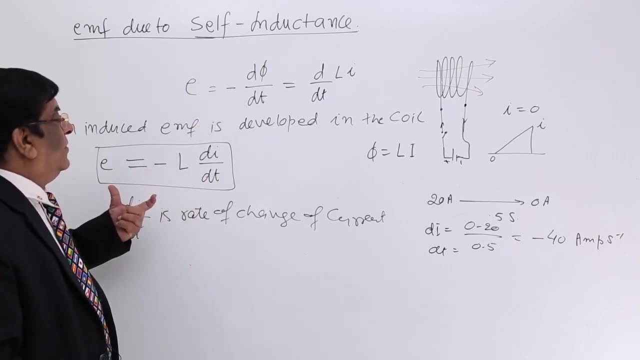 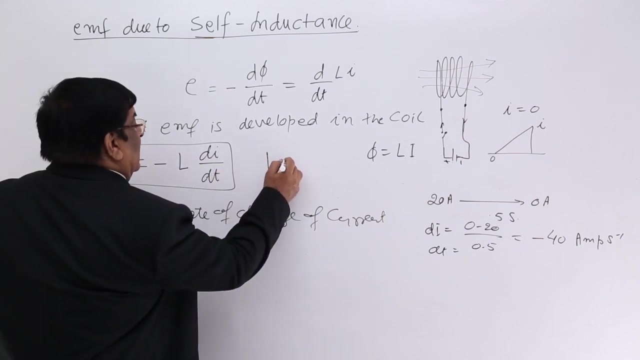 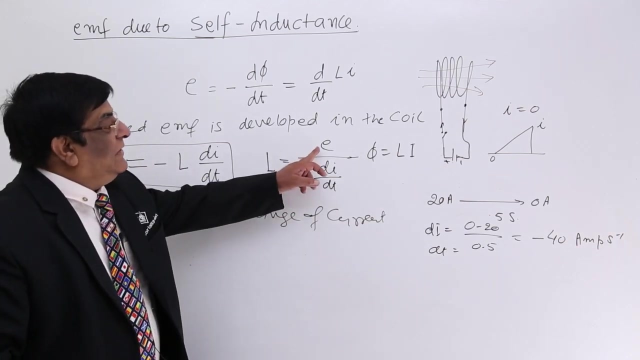 induced EMF which is across this coil. So this is EMF induced across the coil. Now we can define again this self-inductance with help of this E. How much is L here? L is equal to divided by di, by dt in magnitude, and let us leave aside the direction. So L is equal to. 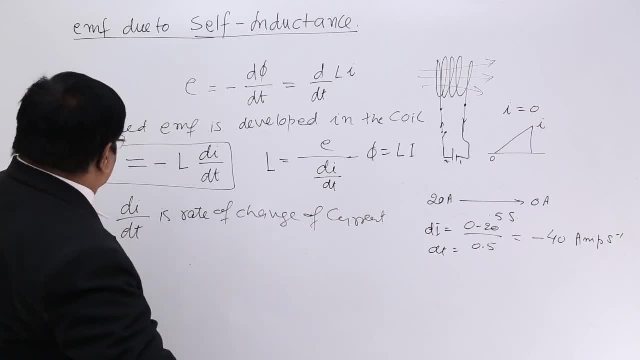 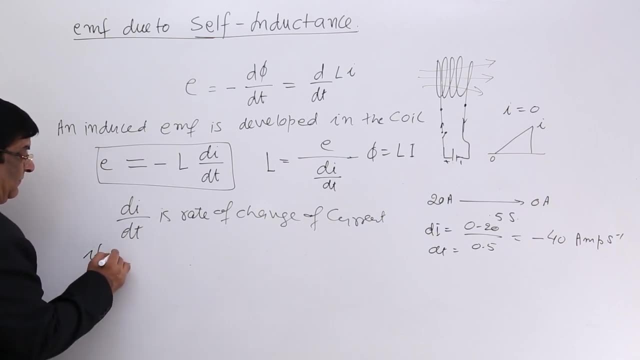 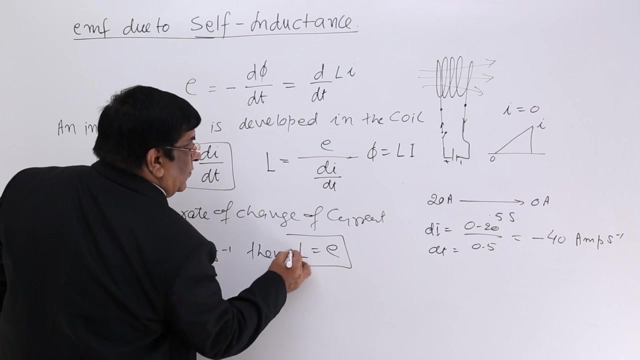 emf induced divided by di by dt. Now if I make this di by dt equal to 1.. If di by dt is equal to 1 ampere per second, then L is equal to E. What is E Induced emf? Now we 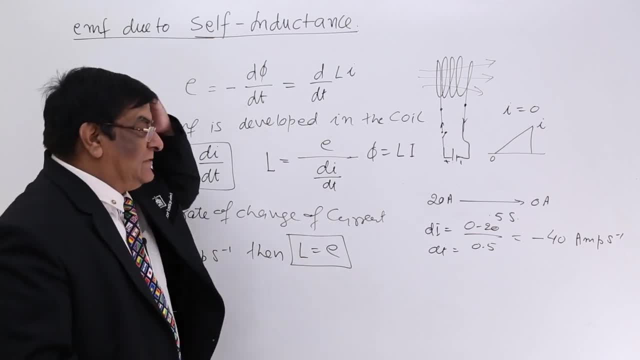 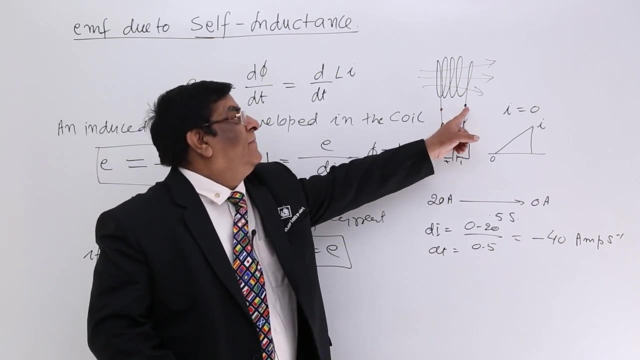 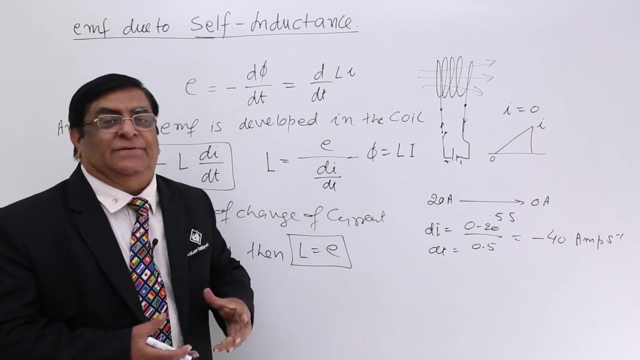 get another definition of coefficient of self-inductance. Coefficient of self-inductance is equal to induced emf across a coil, Because emf is induced across a coil. So emf, or the voltage, is a physical quantity. we can measure Current, we can measure time. 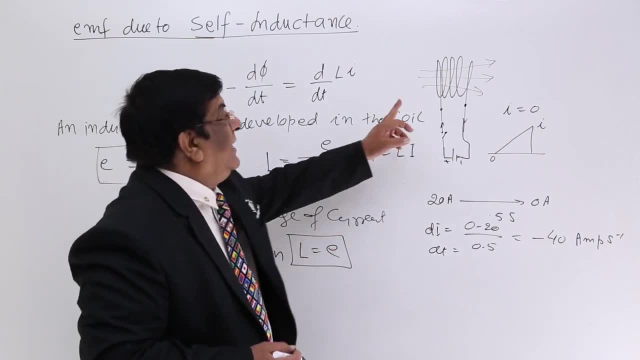 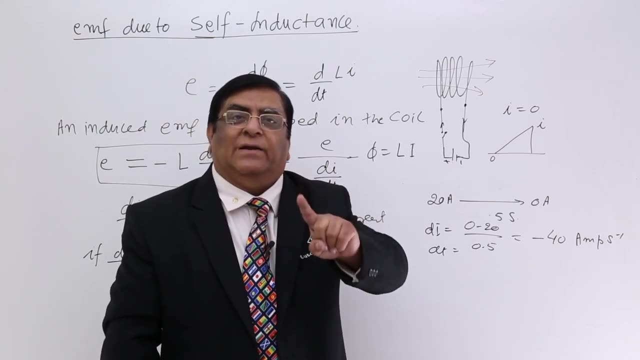 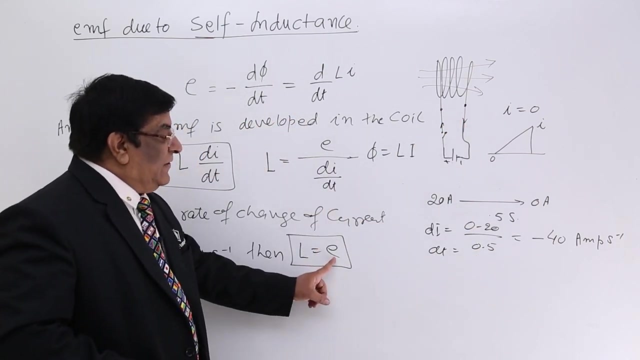 we can measure So in a coil. we take a change of current of the rate 1 ampere per second, Then whatever is the emf induced, whatever is the emf induced, that will be numerically equal to self-inductance. 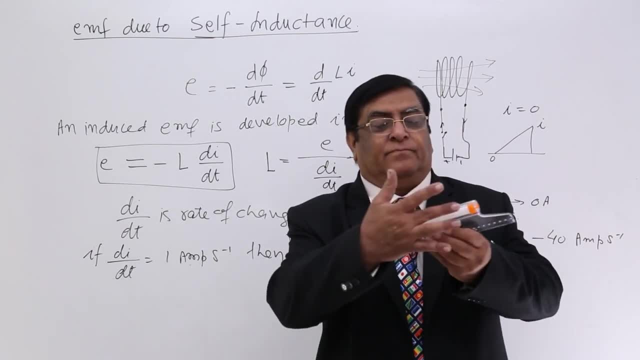 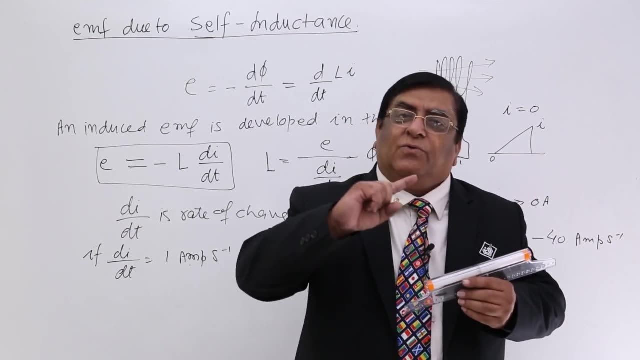 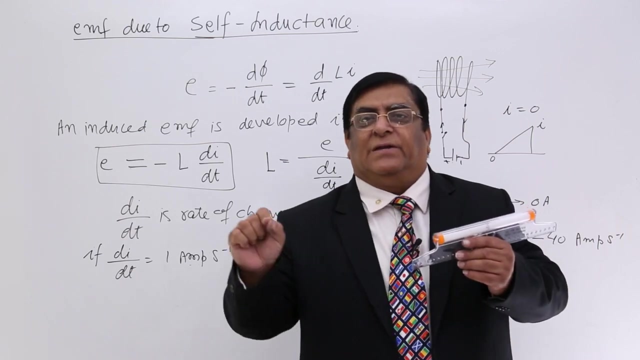 Okay, We have a coil here. in this coil the current is 5 ampere. okay, current are zero. we make it five ampere and we take five seconds by raising it. So current was zero ampere. slowly we increase the current to five ampere in five second. what is the rate of change of? 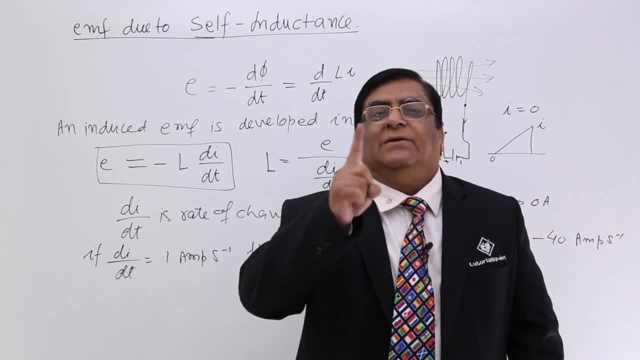 current 5 ampere in 5 second. that is 1 ampere per second. 1 ampere per second. So the Friday's Station. no point reduce the specific λ in this AC square chain for each six second. So each number for each second is equal to ligne. So that was quite the comparison of. each ampere of current for each second. okay, Then we can of course multiply with some or the other. Here it is value of current number 5 for each second, So it is 1 ampere per second. that was very good. evaluation by fluid- CHA2A2C. 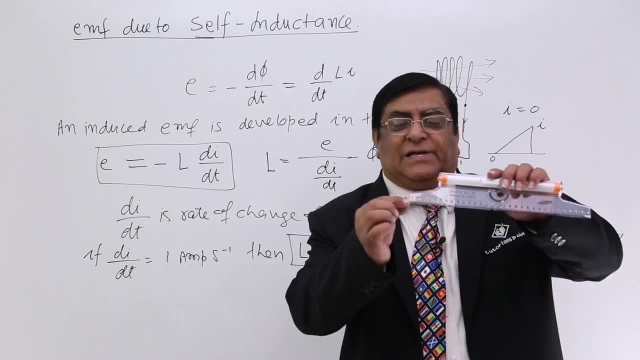 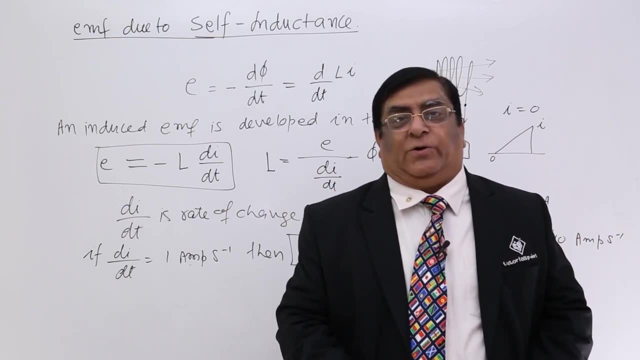 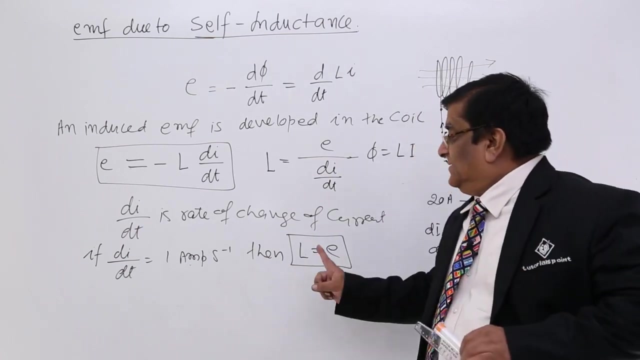 per second. Then what we see across the ends of this coil: a voltage is generated. We measure that voltage. that voltage, 40 volt. 40 volt is generated. If this is 40 volt generated, we say this coil has self inductance of 40 henry. ok. 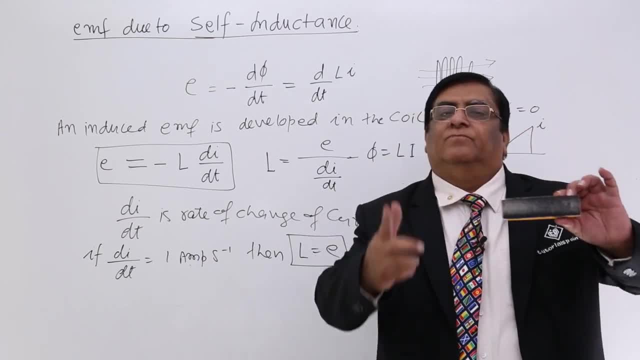 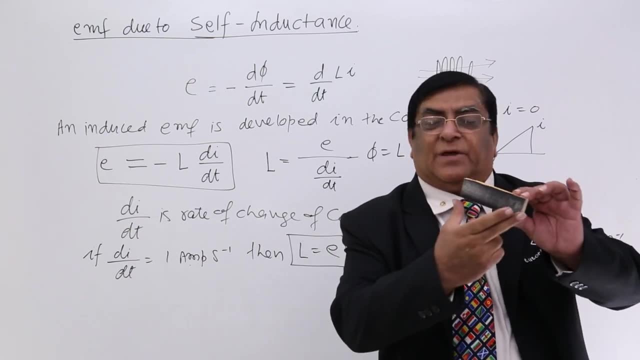 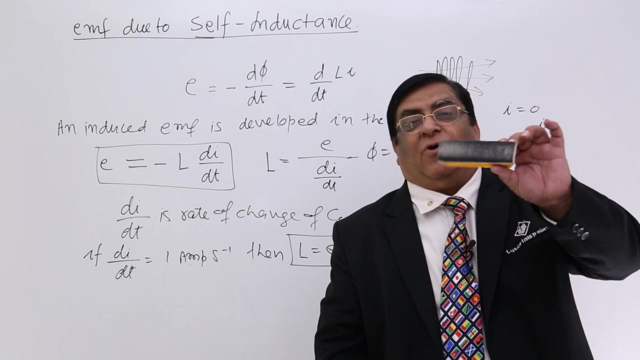 We take another coil, more numbers, more. so again we give it that variable current 1 ampere per second, and during that change 1 ampere per second change. we measure the voltage. here this voltage is 100 volt. We say: this is a good coil, it has got self inductance equal.